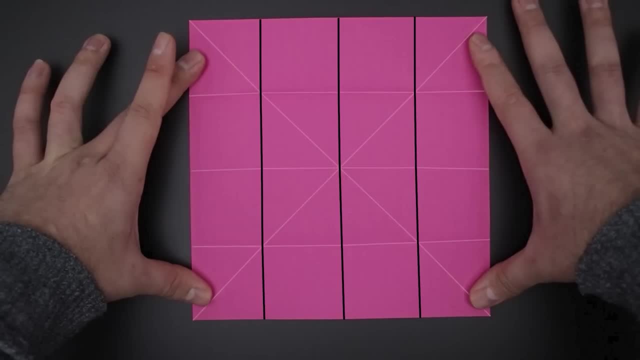 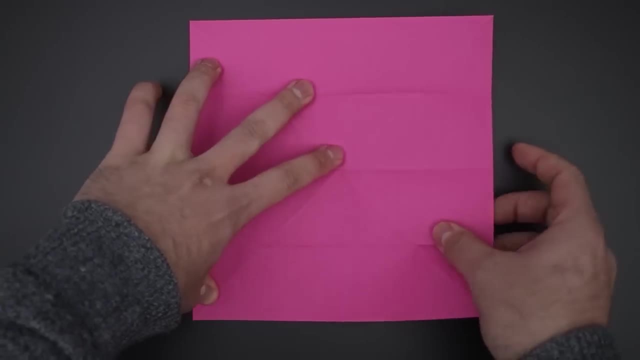 and bring both sides to the middle, making something like necks. So bring both sides to the middle and bring both sides to the middle, making something like necks. So bring both sides to the middle and bring both sides to the middle. 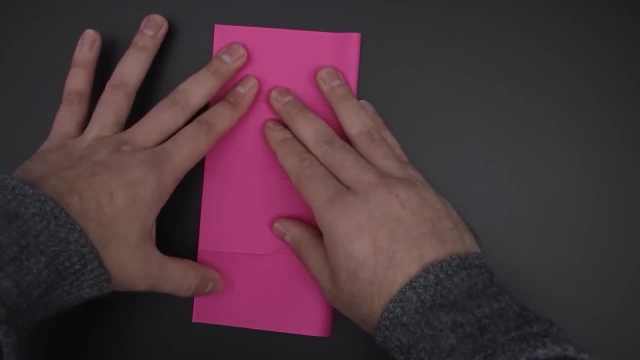 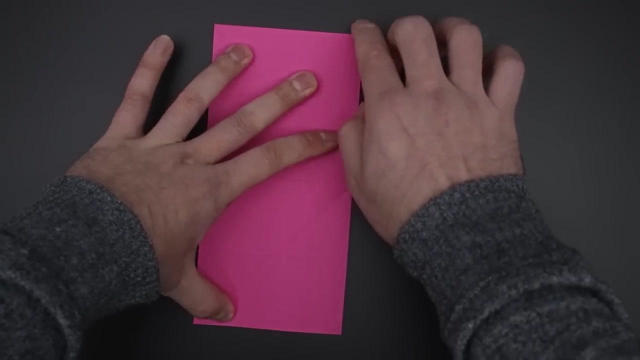 making something like necks. So bring both sides to the middle making something like necks. We will now make the other unlock piece and let go and step back a little bit. So continue folding in two creases with the contact andosition multiplier. 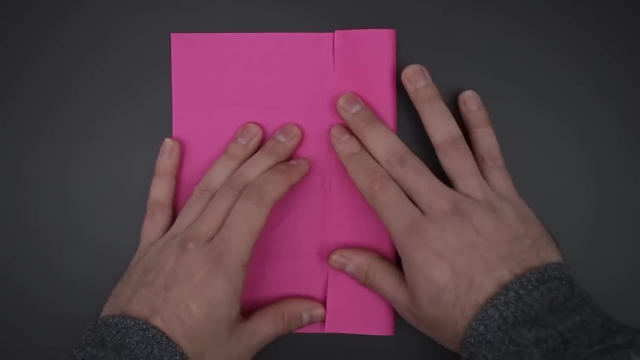 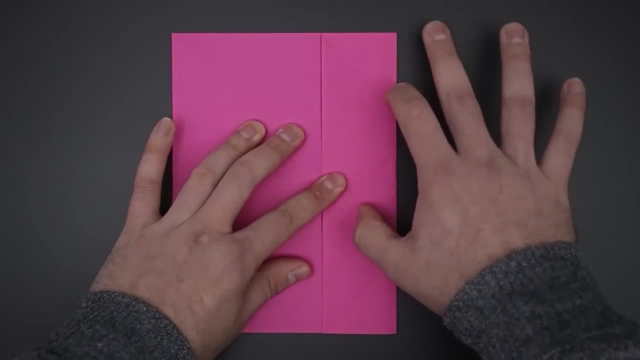 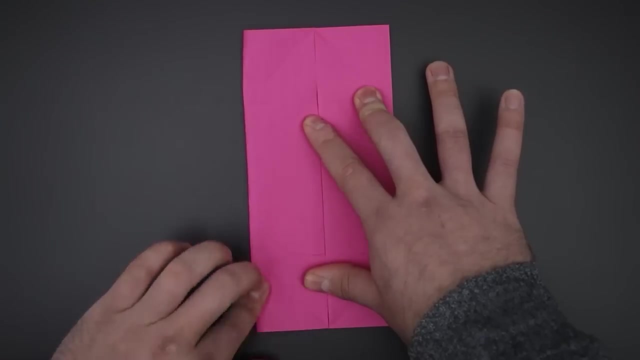 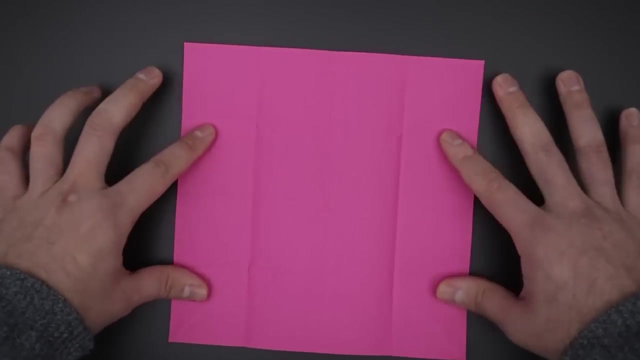 then focus it and see how well you see the intersection, as we'll be covering it in a few moments. Let suit the indicates into the stickers and clean up the areas that see the holes in the connectors. Click the Next button. at this point we'll have to fold diagonally the four squares of the. 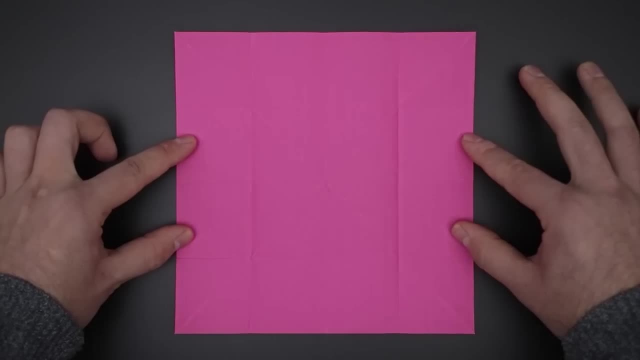 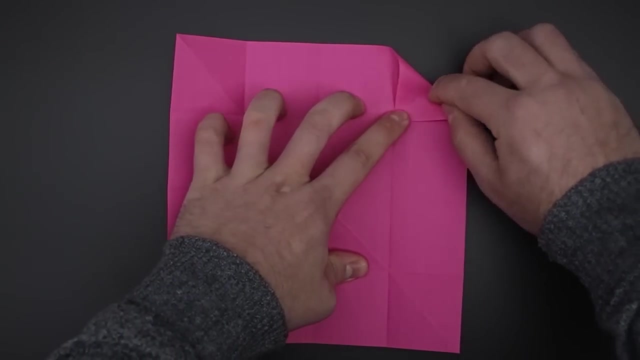 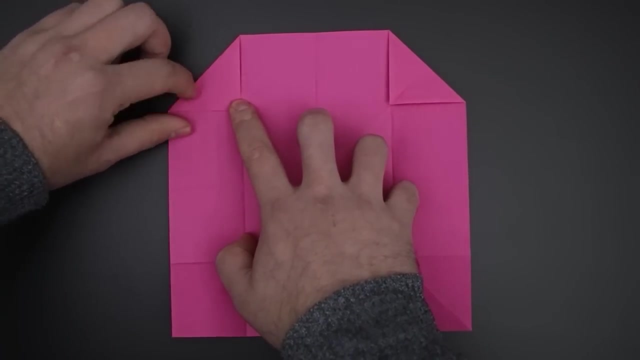 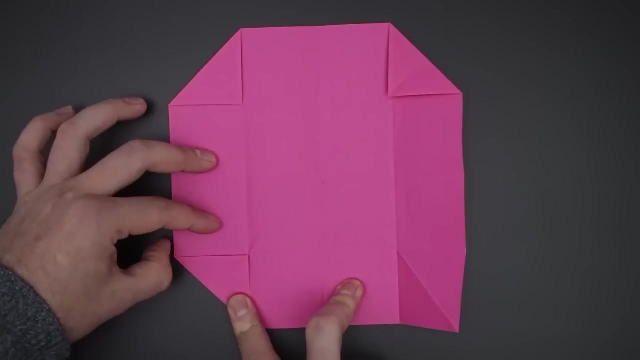 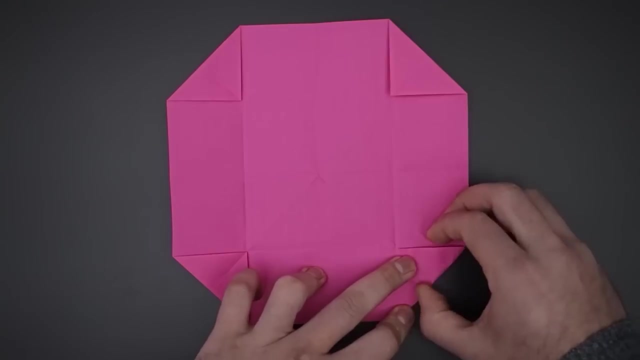 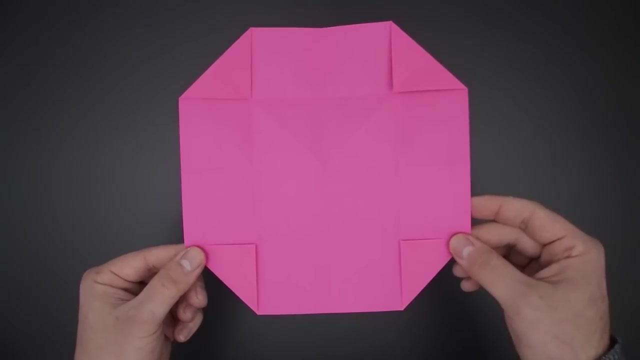 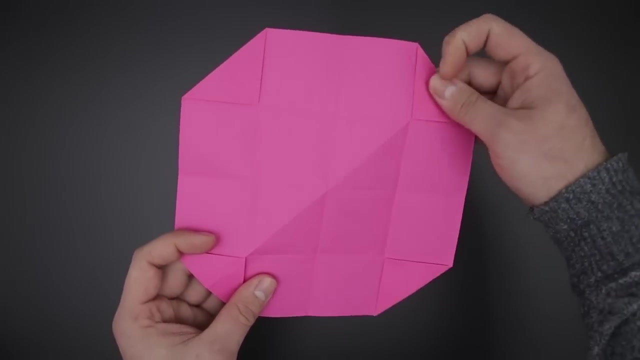 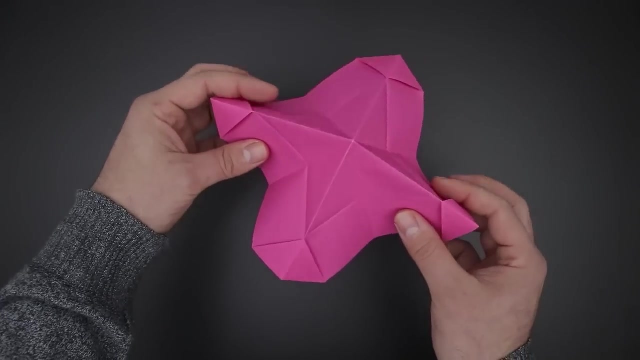 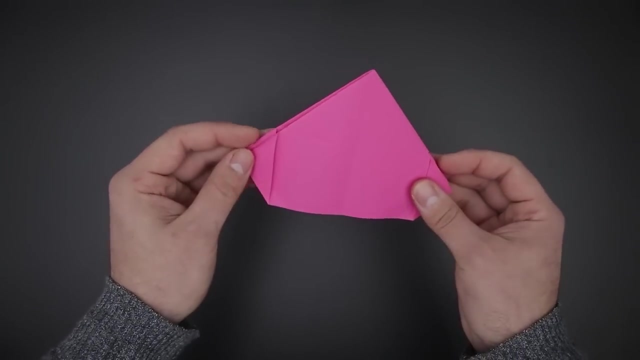 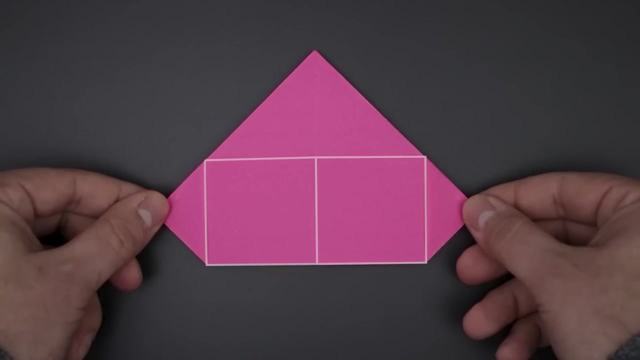 corners. now pay close attention to the next step. we will need to close the paper using these four diagonal folds. to make it easier, you can close the corners first, like this, then just bring the four sides to the middle, keeping the paper in this position down. here we have these two squares. we're 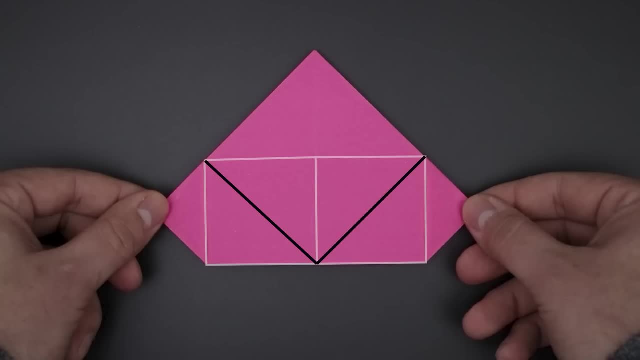 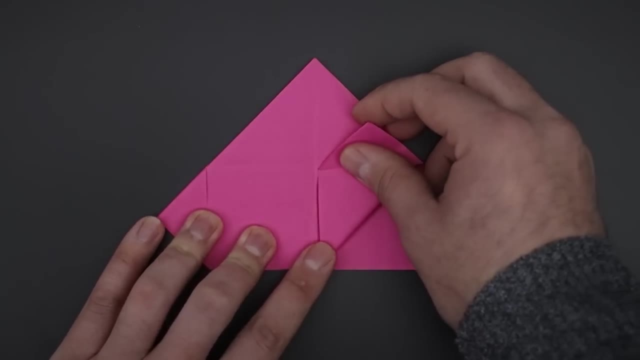 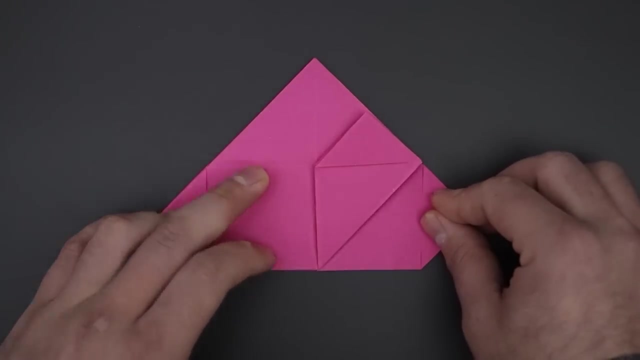 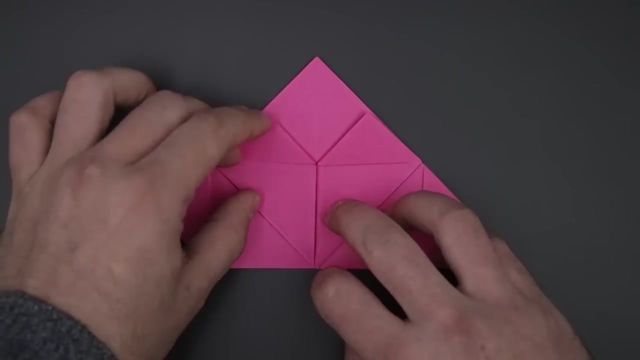 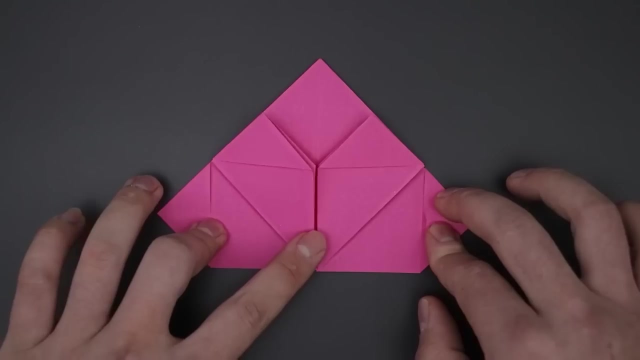 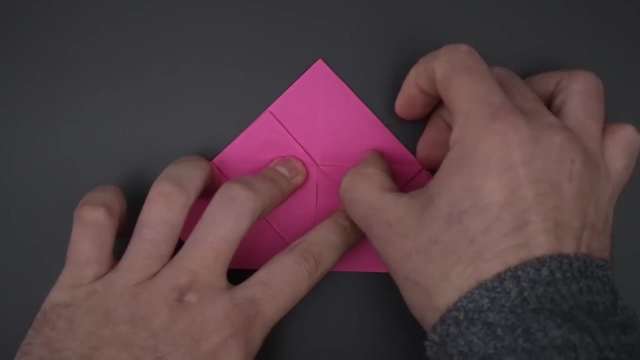 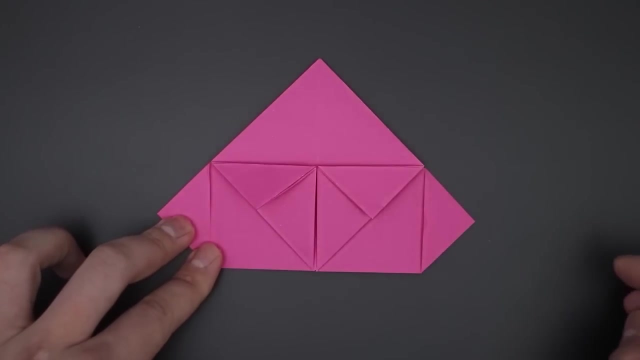 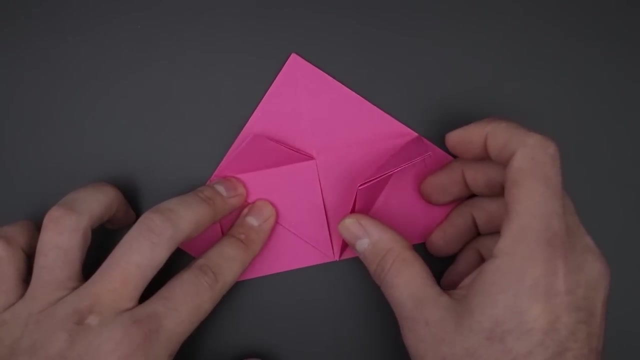 going to fold them both in half diagonally. we can start on the right side, just bring the bottom edge to the middle and reinforce, now repeat on the other side. next, we're going to bring down those triangles that are on top unfold. now, using the marks we just made, let's open one of the flaps and fold the. 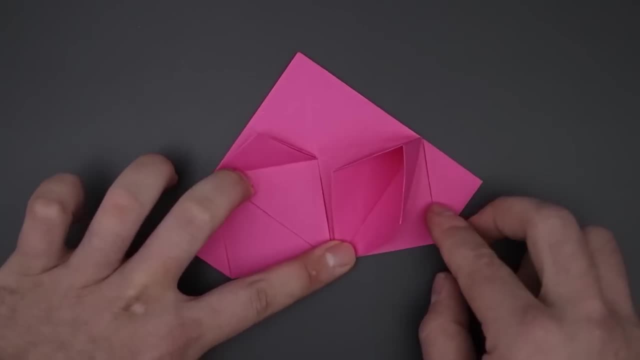 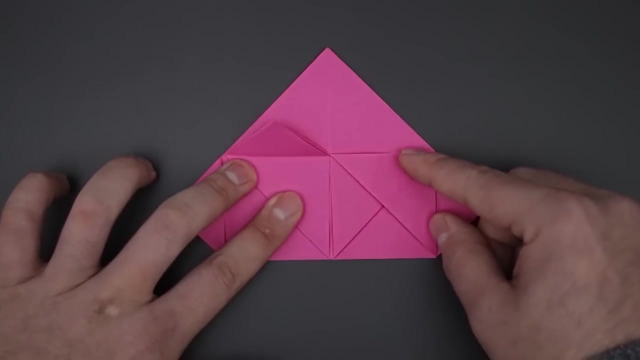 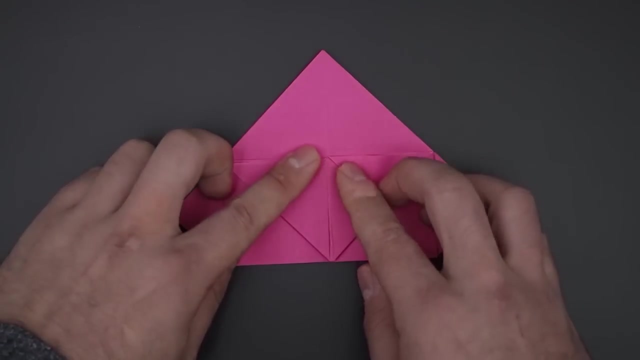 paper and fold it to the middle again. as you can see, i started folding the paper in two halves. we're going to fold these two dick loops in half now. we're going to fold it to the center and fold it in half. now we're going to fold the four sides together. 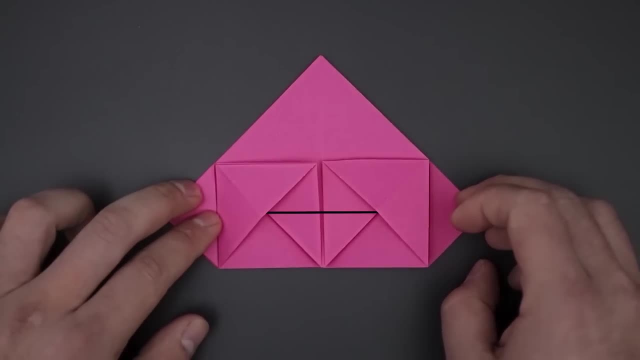 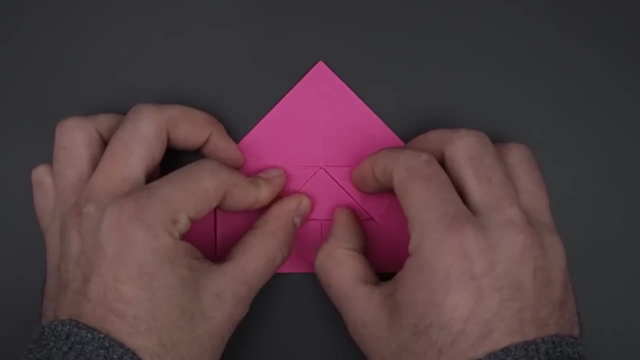 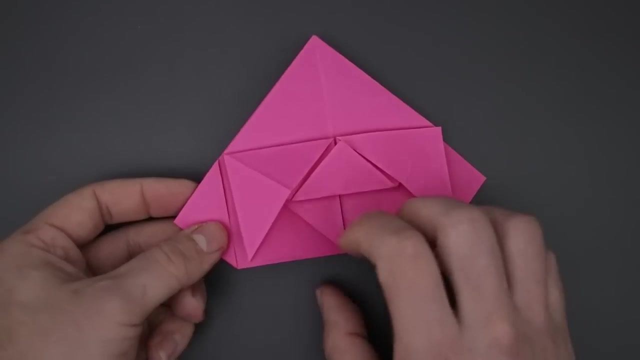 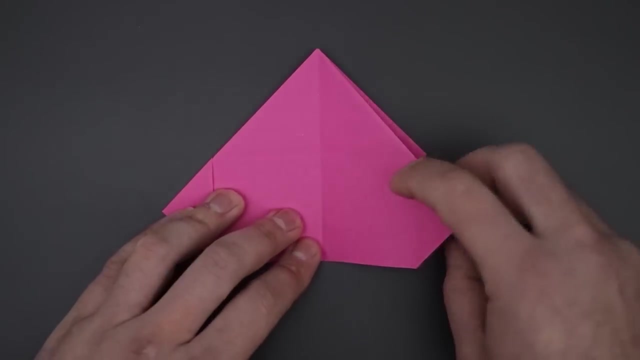 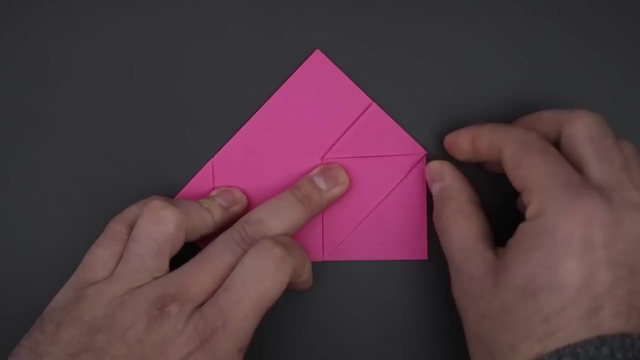 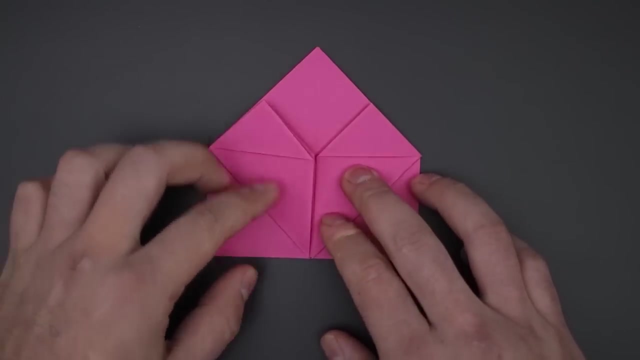 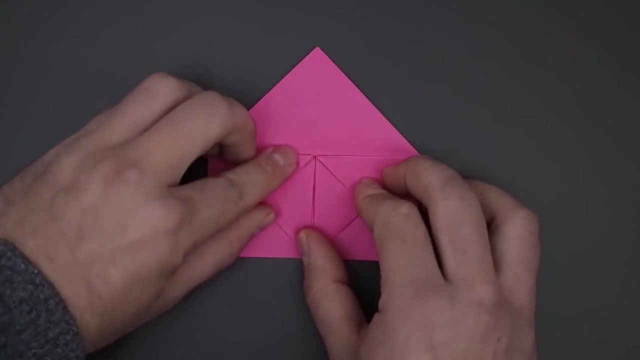 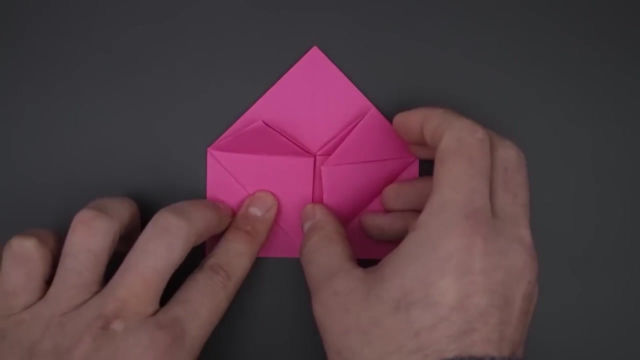 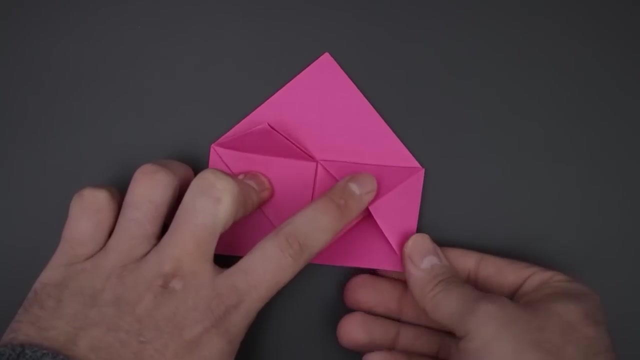 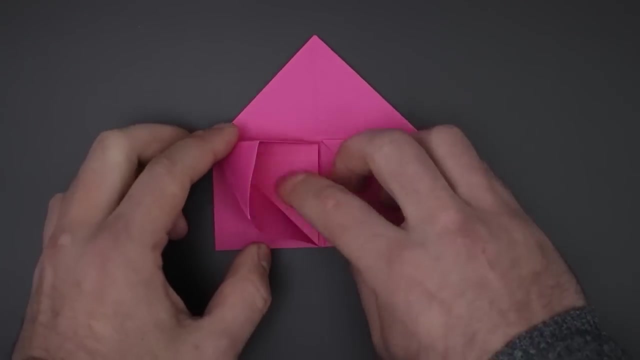 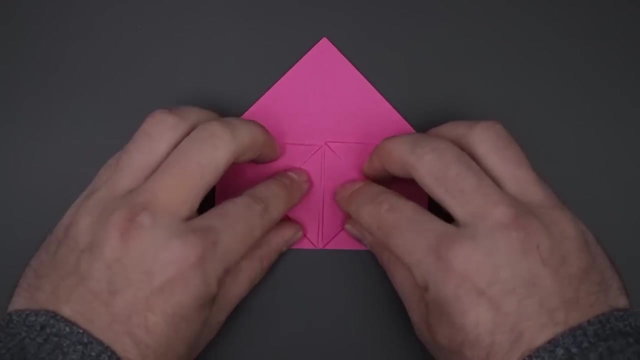 repeat the same process on the other side. And for now this side is ready. let's turn it over and repeat the same on the other. First, we fold the two squares, then bring the corners down, open and flatten. Lastly, we just need to fold the middle corner up. 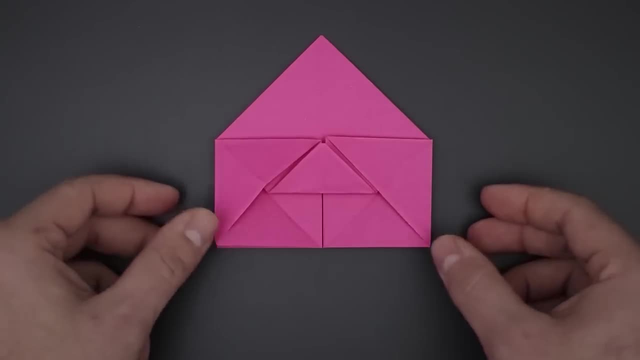 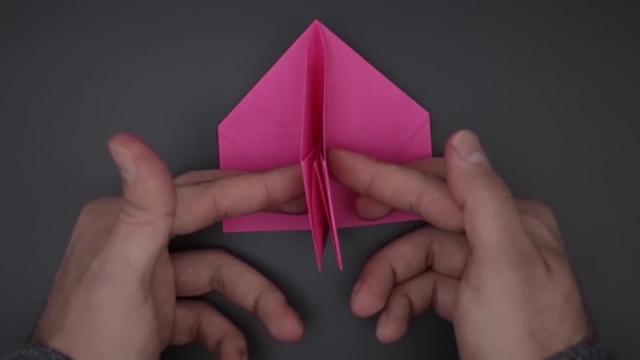 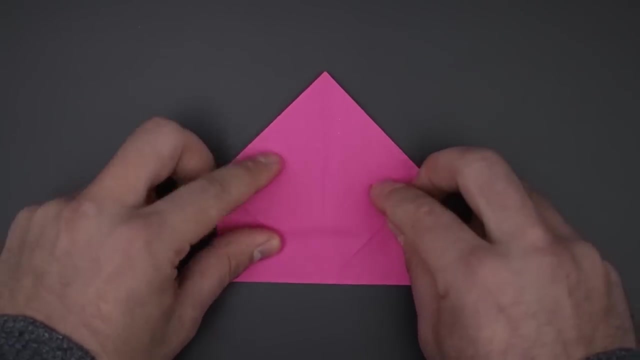 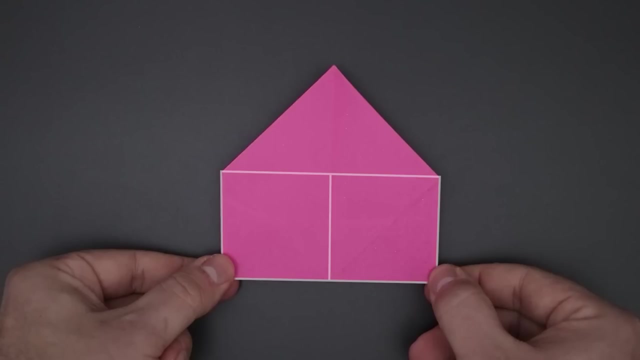 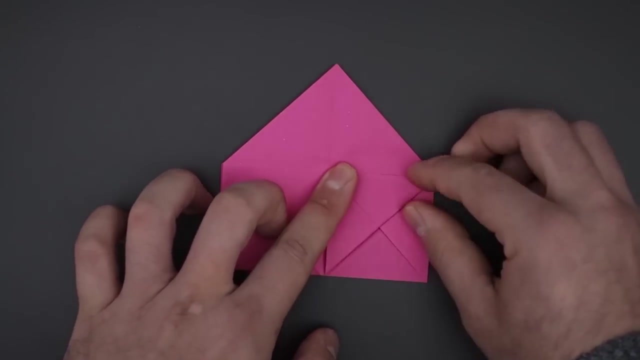 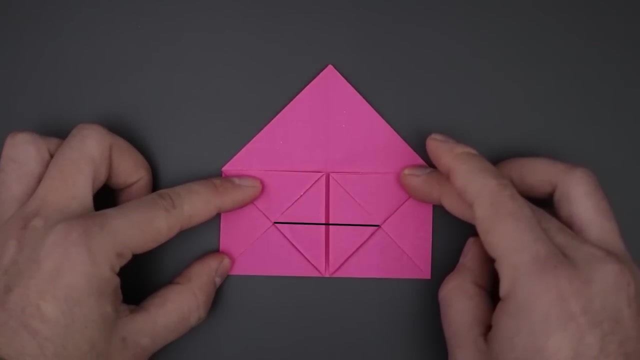 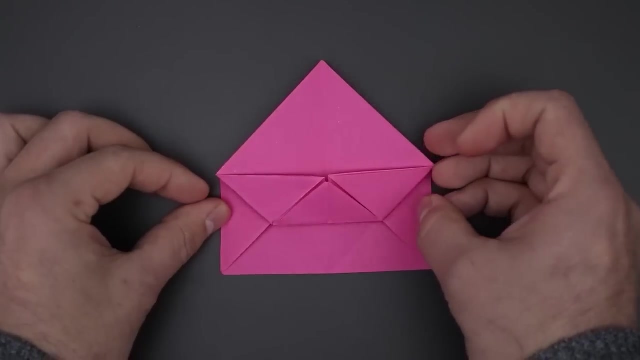 This side is also ready To make the other two. let's first close the front and back sides, And now, with these sides open, let's again fold the squares in half diagonally, And then fold the remaining corner up. Let's turn it over again and repeat with the last one. 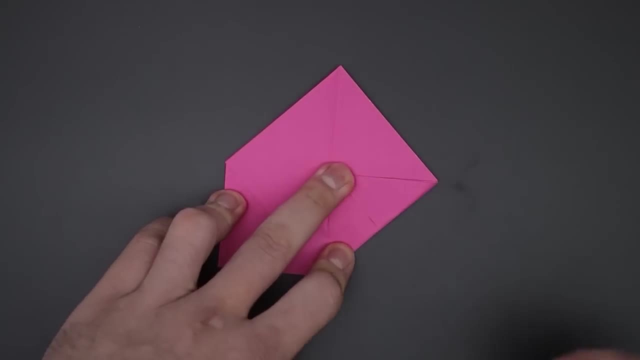 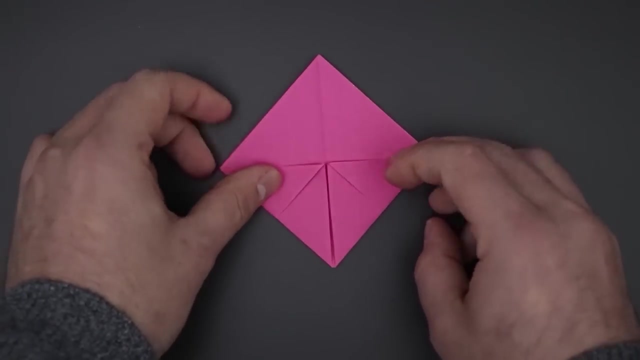 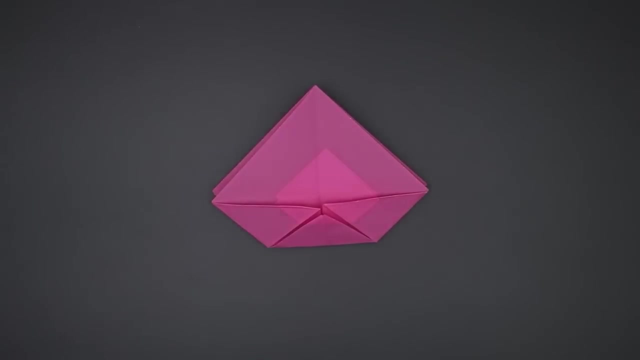 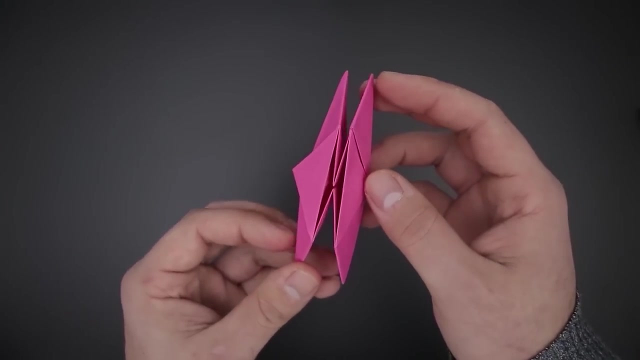 And now, with these sides open, let's again close the front and back sides. Now for the next step. again, pay close attention. If you did everything correctly, you should have something like this Down here we have this small space. We'll have to open this same space by pulling the sides of the paper. 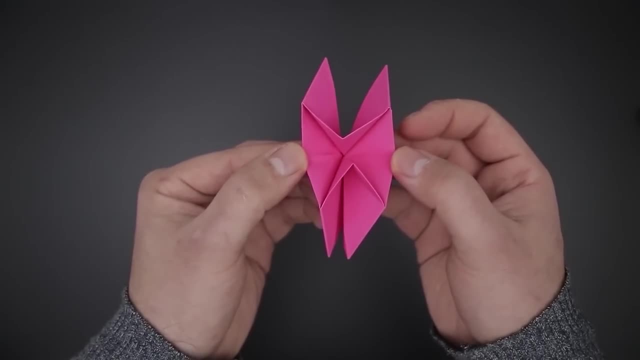 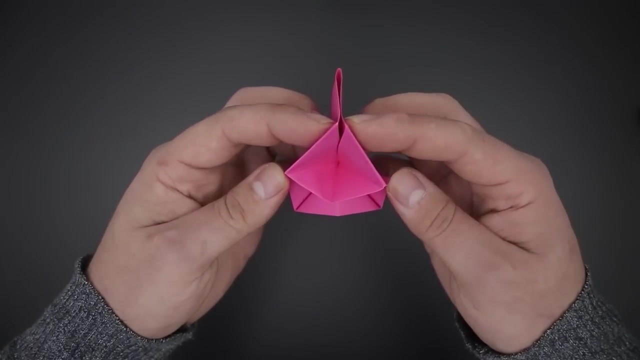 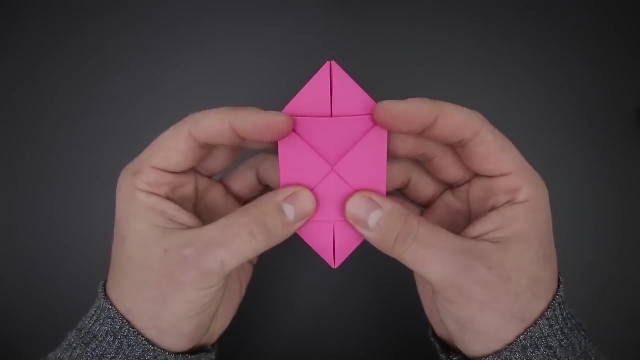 We'll have to open this same space by pulling the sides of the paper. We put the top and bottom sides together too. We put the top and bottom sides together too, And mark the middle part. very well, shaping these triangles. And mark the middle part. very well, shaping these triangles. 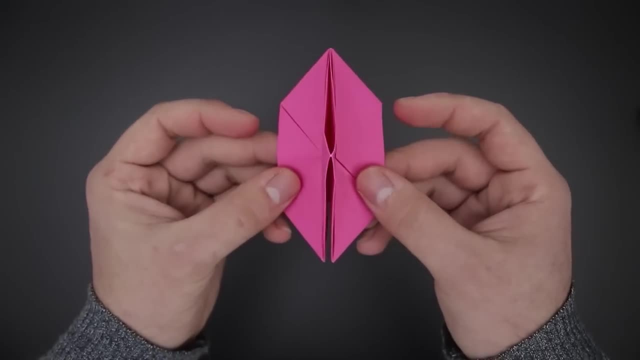 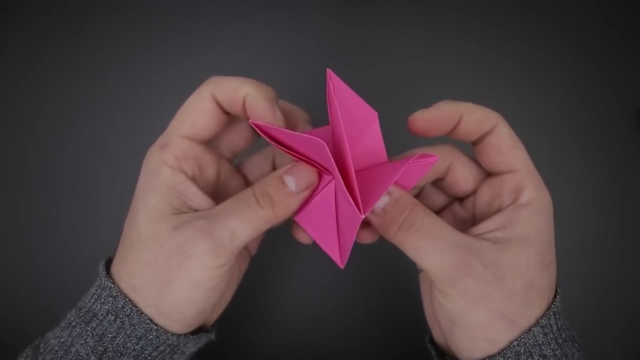 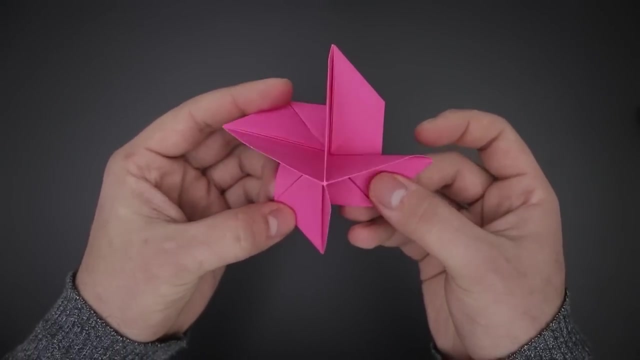 Now, going back to the other side, we have these four flaps. We'll have to open them, leaving each one to one side, Something like a propeller or a ninja star. Now to make the first details of the rose. 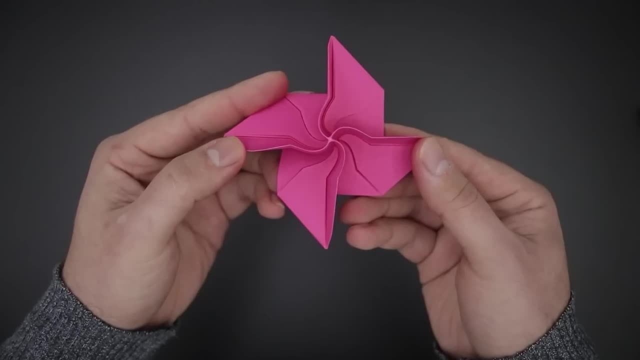 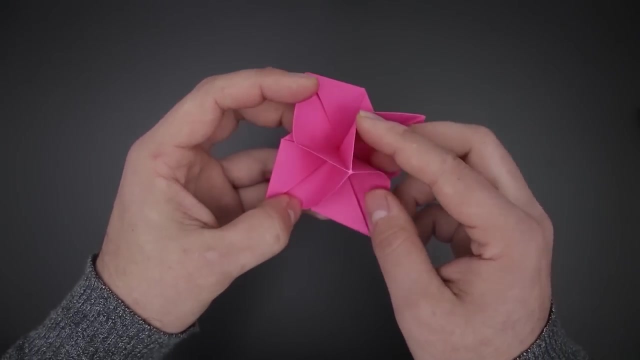 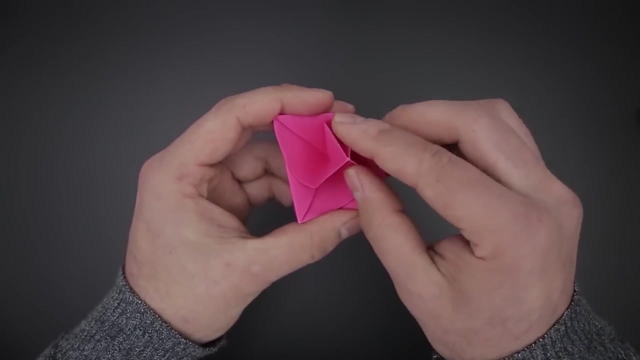 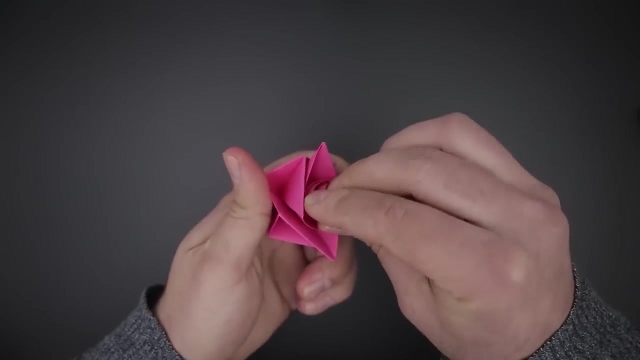 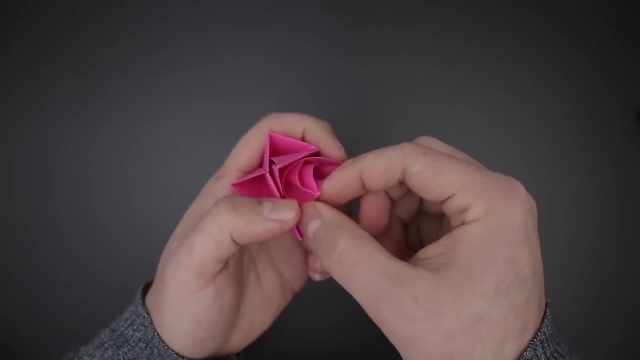 we're going to have to rotate the paper in the middle, creating something like a spiral. Just bend each side following the same direction of the previous step. Just bend each side following the same direction of the previous step. After releasing, this is the result. 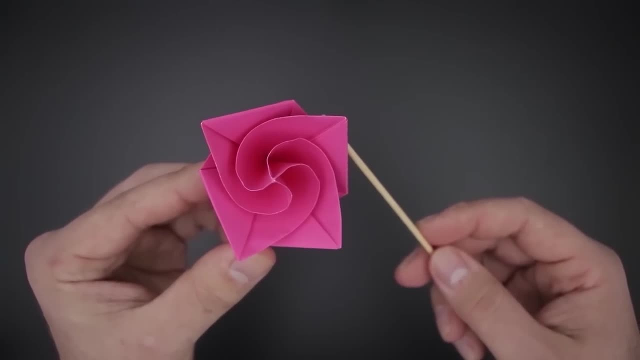 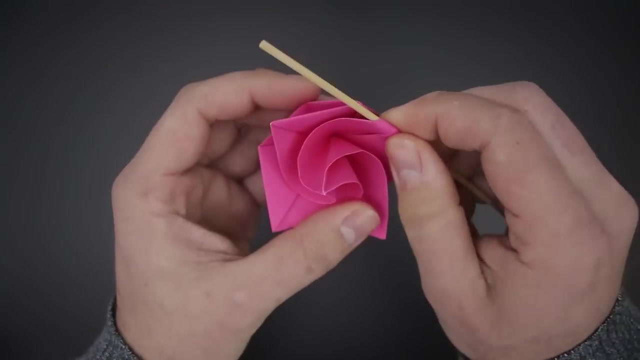 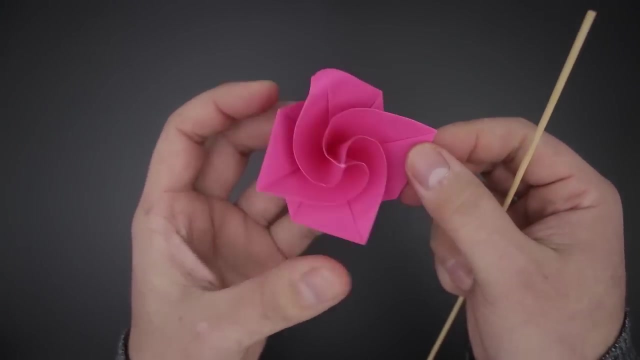 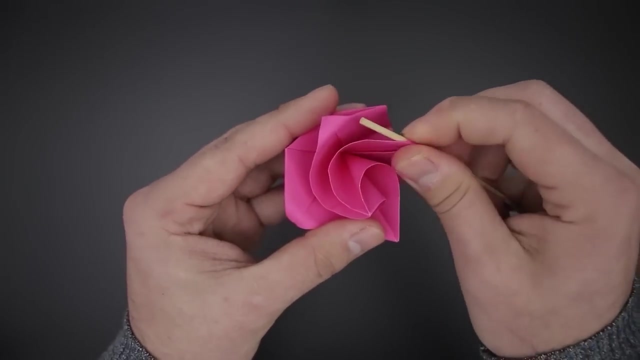 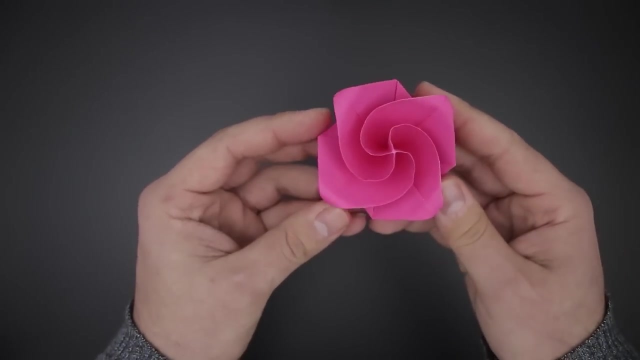 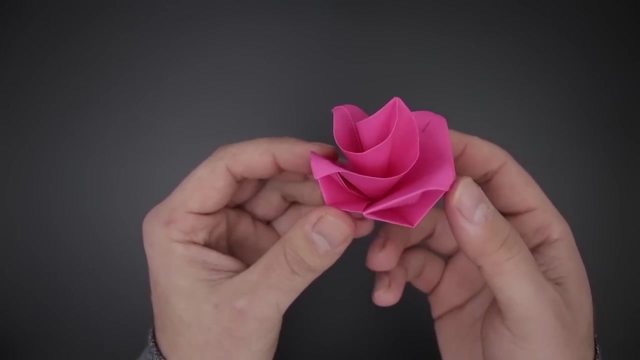 To make it even more beautiful. we can also bend the corners of the petals To make it even more beautiful. we can also bend the corners of the petals, And our Origami Rose is ready. I really hope you enjoyed this video. if yes, remember to click like and also subscribe. 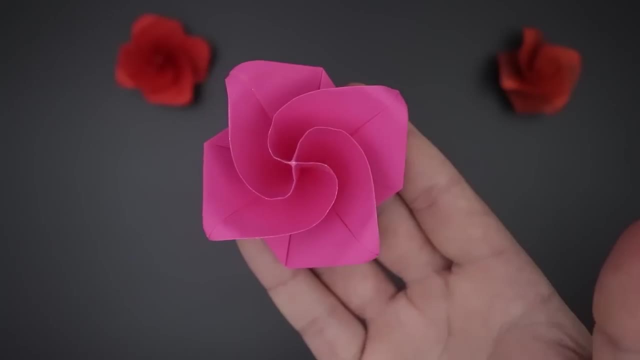 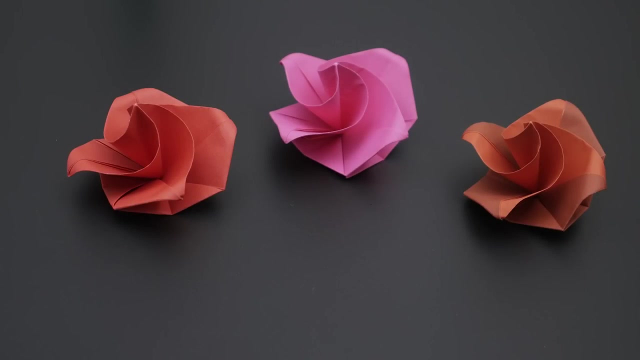 to my channel. Thank you very much for watching. see you next time. Bye, bye.